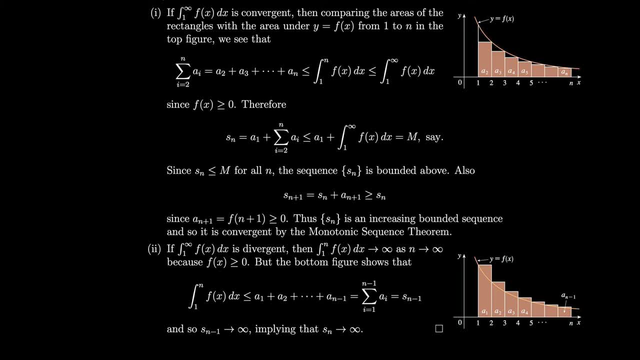 the area of each of these rectangles. then the area is just the height of the curve times the width of the rectangle, So the height of the curve. well, we're doing some right rectangles. so that means that the height will be the value of the function at the integer on the right side. 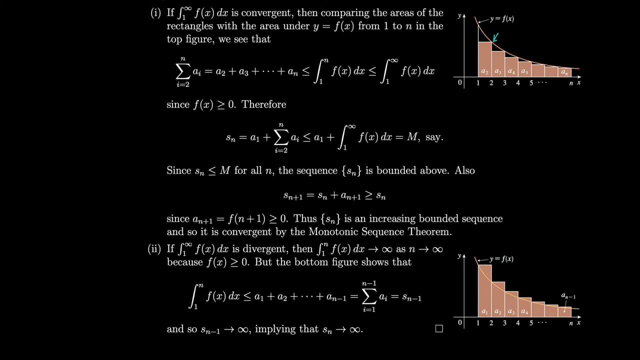 of the rectangle. So that means that if we want the area of each of these rectangles, then the first rectangle we're looking at the right side, which will be at 2.. Second integral will be at 3, the fourth at 4, and so on. So that means that this rectangle has an area of the value of the. 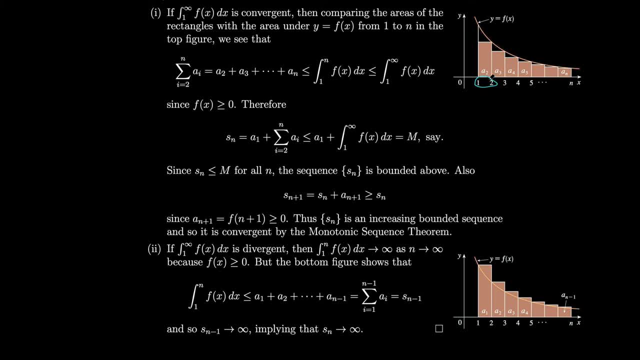 function at 2,, which is a2, times the width, which is 1.. So it's just an area of a2.. And the next one has an area of a3, an area of a4, an area of a5, and so on. So that means that if we add up all of 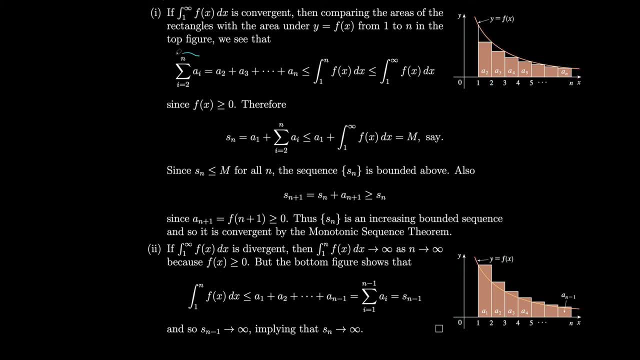 these areas. then we get the sum Of all of these a. i's starting at 2.. So that must be less than or equal to the area underneath the curve, which is the entire area, because look at all these gaps in between. So that area 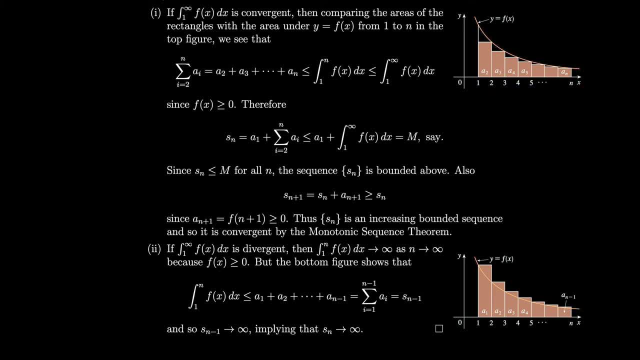 underneath the curve from 1 to n must be even smaller than if we went on forever. So the integral from 1 to n is smaller than the integral from 1 to infinity. so that means that we have this sum from 2 to n smaller than the integral from 1 to infinity, And this is all you know predicated on. 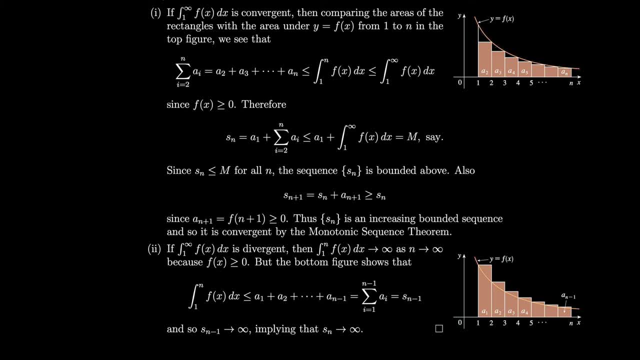 the fact that f of x is greater than or equal to 0, and that we have a decrease in continuous function. Notice, if this function was not going down, then we wouldn't have this underestimate for rectangles, so we wouldn't have this inequality at all. So then we can write that the sum of the 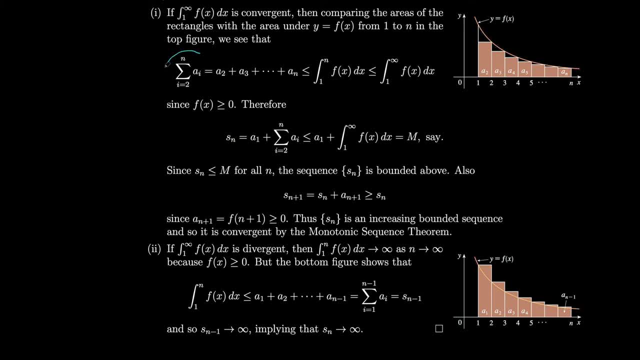 sum in general is equal to everything from 2 on, as long as we just add that initial term that we didn't have. So that must be equal to the integral plus that initial term. We basically just add a 1 to both sides of this inequality over here. So this a 1 plus our integral, because our integral 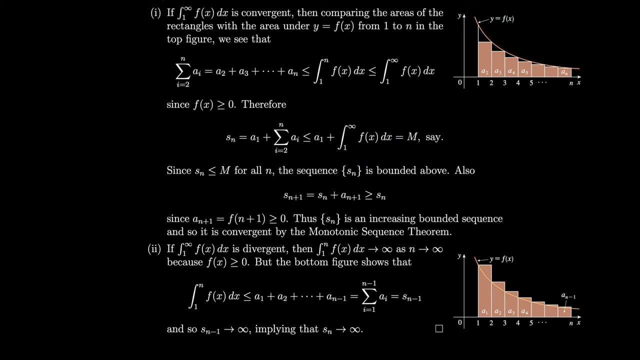 is convergent, it equals some number. So we take that number, we add it to a 1, we get some other finite number. so let's just name that number m. So it means Sn is bounded by m for all n. 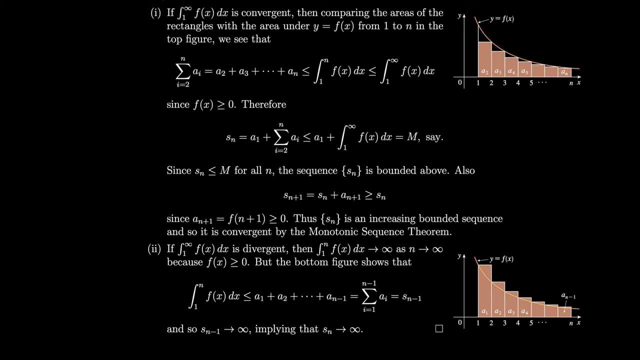 so our sequence is bounded above. But we also know that Sn plus 1,, which is Sn plus our next term, is greater than or equal to Sn, since our An plus 1 term is Fn plus 1, which is also greater than or. 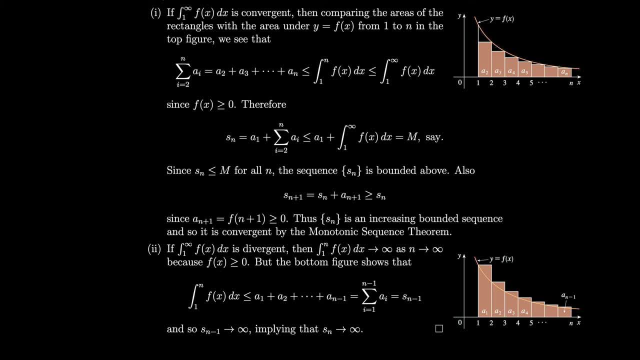 equal to 0.. So we have an increasing sequence and it's bounded, so it must be convergent by the monotonic sequence theorem. So, as a quick example of this, how about we take a look at the possibility that F of x was 1 over x squared? So then this first rectangle has an area of the. 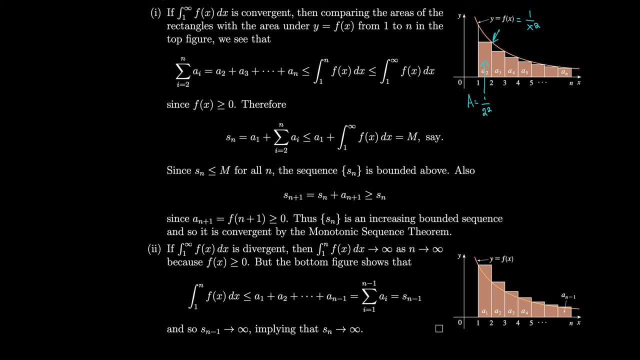 area of 1 over 3 squared and then we have an area of 1 over 4 squared, and so on. So if we take the sum of all of these areas, then we get an under-approximation for the area underneath the. 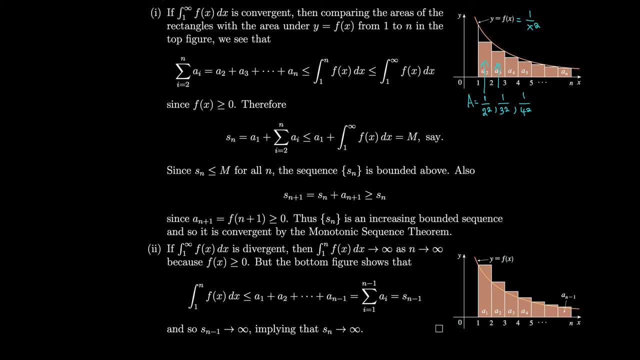 curve. So it makes sense that adding up 1 over 2 squared we get an under-approximation for the area of 1 over 3 squared, 1 over 4 squared. That should all be less than the integral from 1 to. 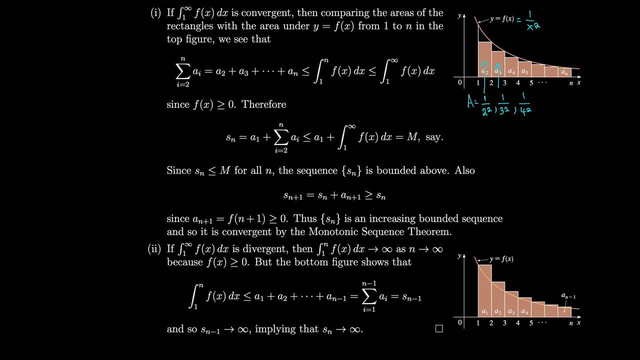 infinity. So if we took 1 over 1 squared- our only missing term in the series of 1 over n squared- we added that to our integral from 1 to infinity of 1 over x squared dx, then we would get 1 over. 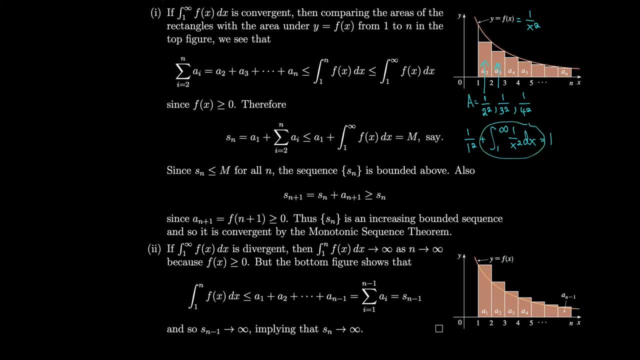 1 squared is 1.. And then this integral we calculated in section 7. 8, we saw that it converges and it's also equal to 1, so then this would be 2.. So that would be the entire area underneath the curve plus the first term that we didn't put. So that means that. 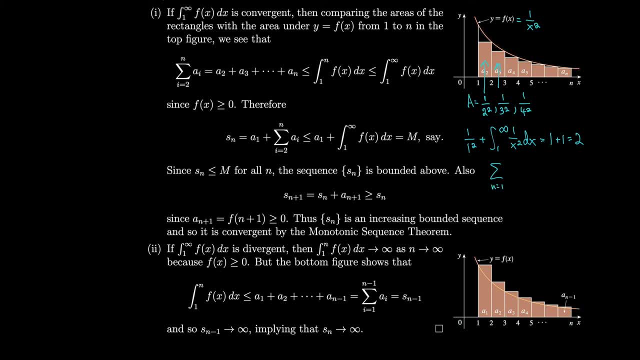 the sum for n equals 1 to infinity of 1 over n squared should be less than 2, because the sum is just the rectangles Without all these gaps. So that must be less than the integral plus the first term. Notice that this does not give you the value of the series. It only tells you that the series 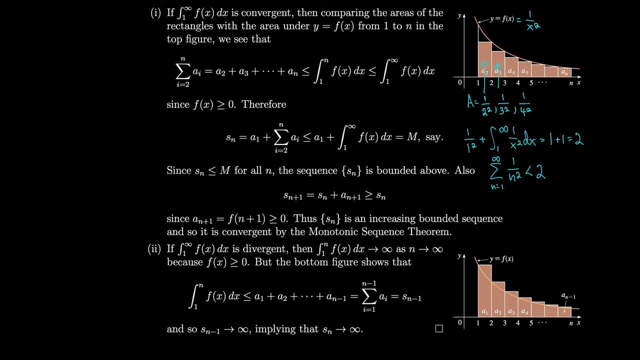 converges. If you actually wanted the value of the series, you'd have to do something a lot more complicated. In this case, the sum of 1 over n squared is actually pi squared over 6, and it's not easy to compute. So the only thing the integral test can tell you, provided that you have a suitable. 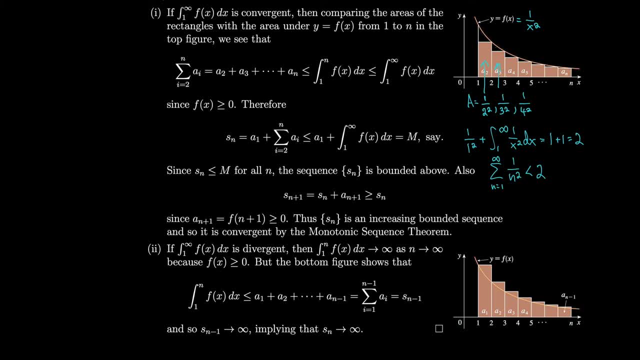 function is whether or not the series converges. Notice that when we did the sum of 1 over n, the harmonic series, it actually diverged, because that actually corresponds to the integral 1 over x diverging. But let's finish up this proof. 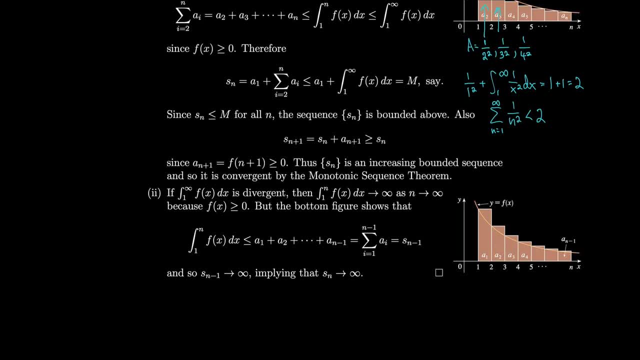 over here. The other case is that the integral is divergent. So in that case our integral from 1 to n goes to infinity as n goes to infinity. So in our bottom figure what we do now is we take rectangles on the left side. 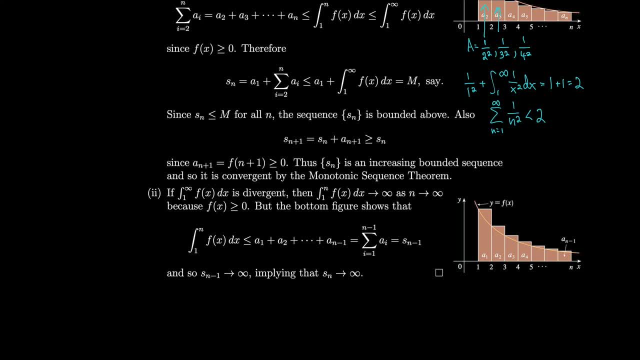 which will be an overestimate for the error underneath the curve. Notice, if we take them at the left side, then our first one starts at 1 instead of starting at 2.. So we immediately get that a1 through an minus 1 is greater than or equal to this integral from 1 to n above x, dx. 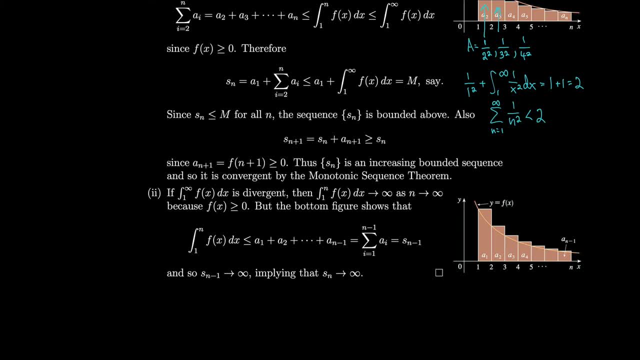 So that means that our partial sum up to n minus 1 already diverges from the integral from 1 to n above x dx. So that means that our partial sum up to n minus 1 already diverges from the integral from 1 to n above x dx. 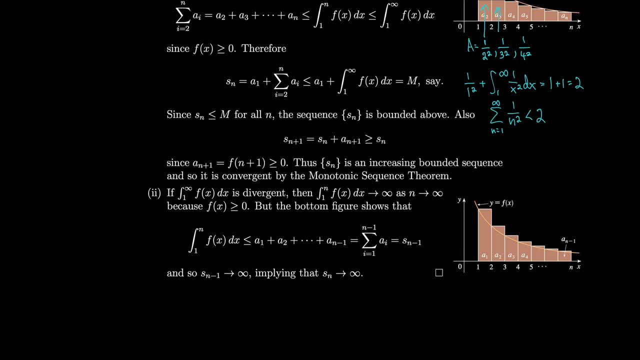 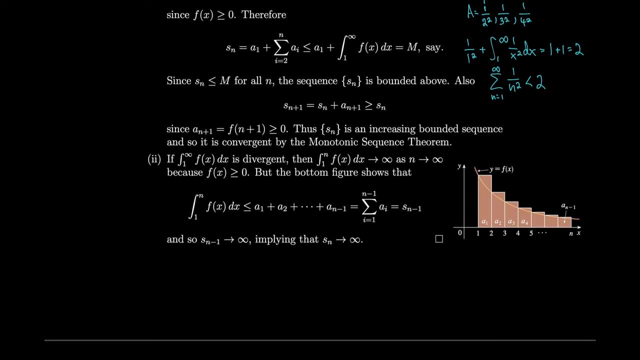 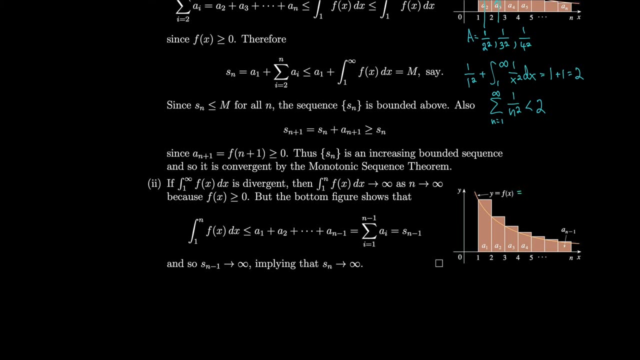 to infinity. So, of course, adding the next term, that an to complete it and gave you sn, is definitely going to cause it to diverge also, which makes it even worse. So, as an example, what we could do is take a look at thewe already looked at 1 over n, so how about we look at 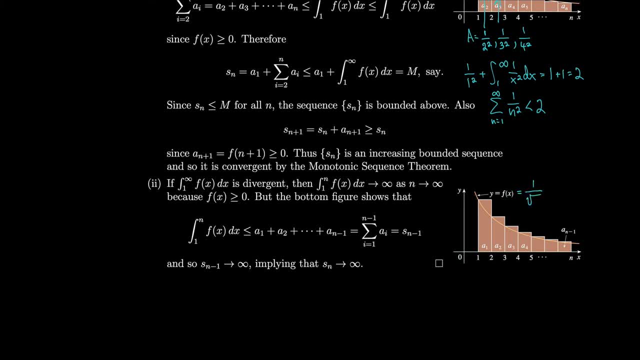 1 over square root of x. So in that case our first rectangle has an area of 1 over square root of 1.. Then we get 1 over square root of 2.. Then we get 1 over square root of 3, and so on. 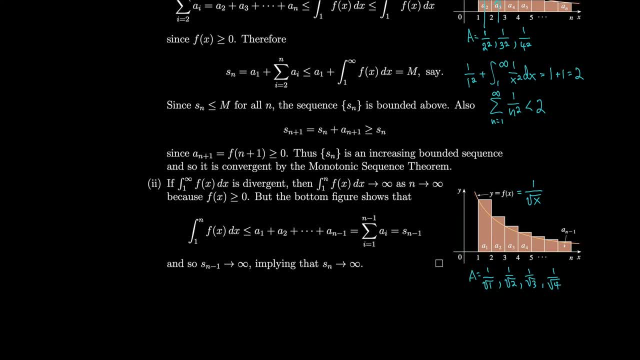 So all of these rectangles over-approximate the area of the curve. We know that the integral from 1 to infinity of 1 over the square root of x, dx diverges, as we saw in section 7.8.. So that means: 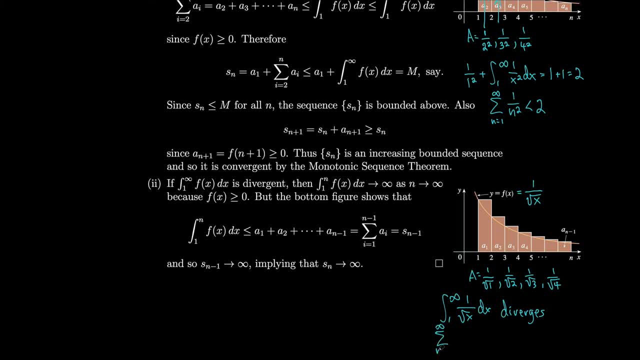 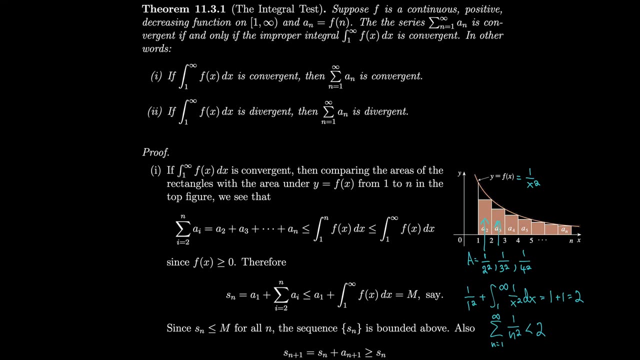 that our sum from 1 to infinity of 1 over square root of n must diverge as well, because it's even bigger. So notice that in order to use the integral test, you need quite a few conditions. You need a continuous function, you need a positive function. 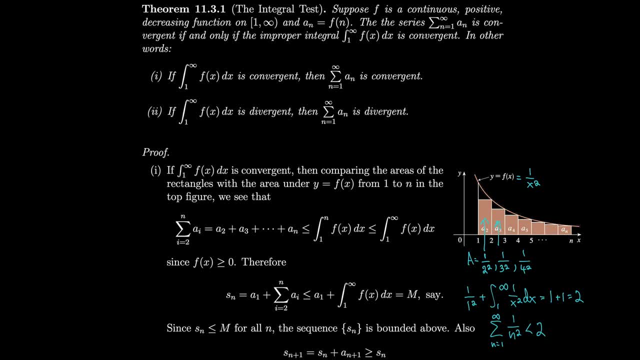 and it needs to be decreasing, and you need a function that corresponds to all of your a? n's. So we can relax this a little bit at least by saying that the function does not actually have to be always decreasing, it just has to be ultimately decreasing. 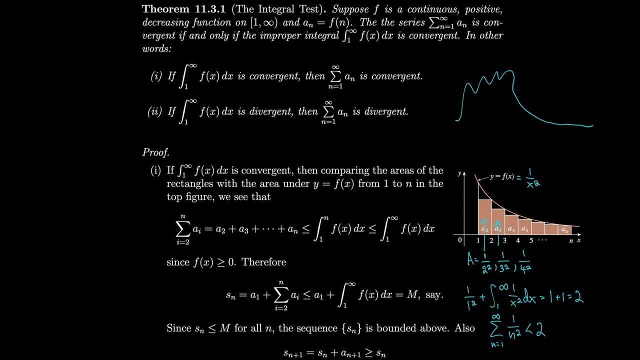 In other words, my function could do something insane as long as it levels off towards the end, And, of course, it has to stay continuous. So instead of saying that it needs to be decreasing from 1 to infinity, I could use any number past 1 as well. 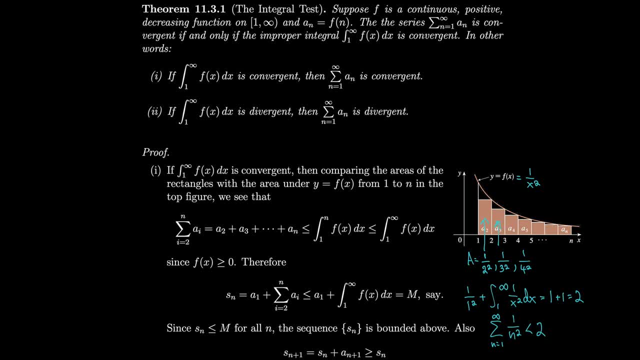 This follows in the fact that we talked about in the previous section, where if you have a a bunch of finite terms in a series, those finite terms at the beginning of the series don't really matter so much. they don't really affect the convergence of the series. 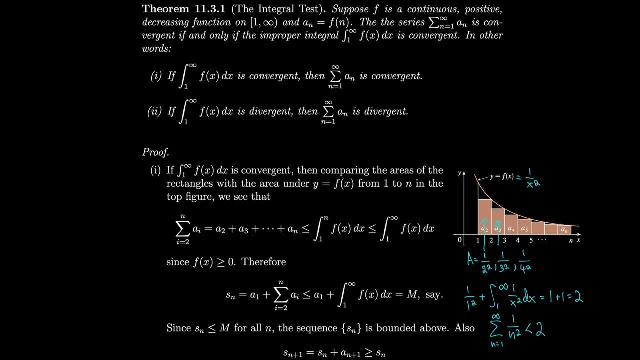 If your series converges after a certain number, then it'll converge. if you throw in a couple extra numbers, It'll change the value, but it won't affect the convergence or divergence. So we'll do a couple examples where we start a little bit past 1. 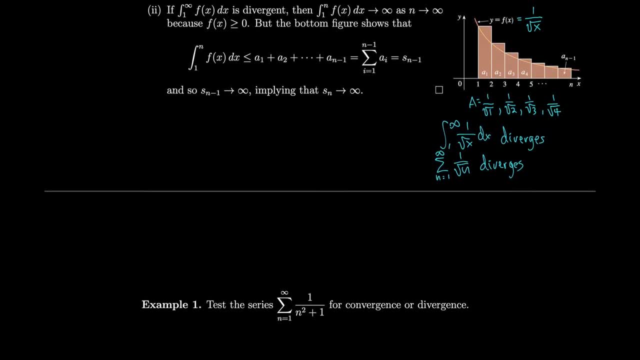 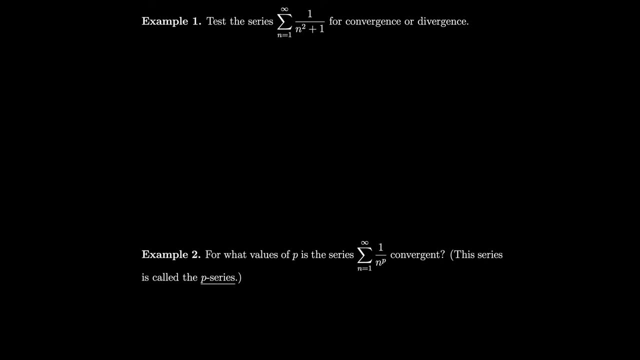 with decreasing functions. Let's start by testing the series 1 over 1 over x squared plus 1 for convergence or divergence. So we need a corresponding function. Let's look at: f of x equals 1 over x squared plus 1.. 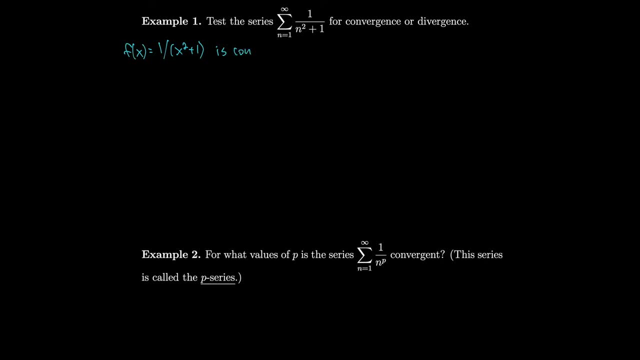 Well, that's definitely continuous positive because of the square and because we're starting at 1. And it's decreasing, And it's decreasing, And it's decreasing, Provided that we are, Provided that we are on the interval. 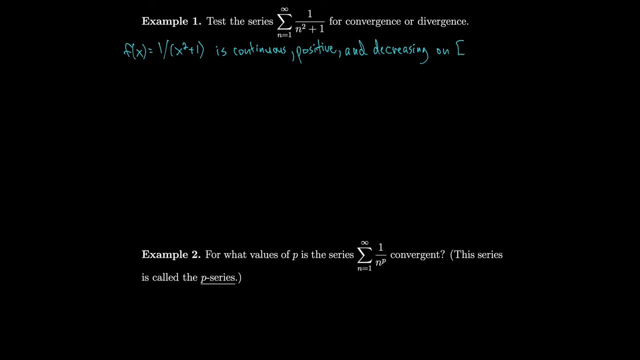 on the interval from 1 to infinity, from 1 to infinity, from 1 to infinity. So let's also take a look at our integral. We need our other condition, where something happens to our integral, And we'll take a look at. 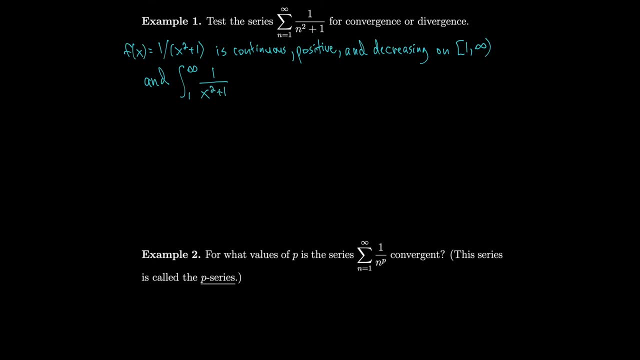 1 over 1 over x squared plus 1 dx as we integrate from 1 to infinity. So remember that for improper integrals we're taking the limit as some other variable goes to infinity, where we insert that variable instead of infinity. 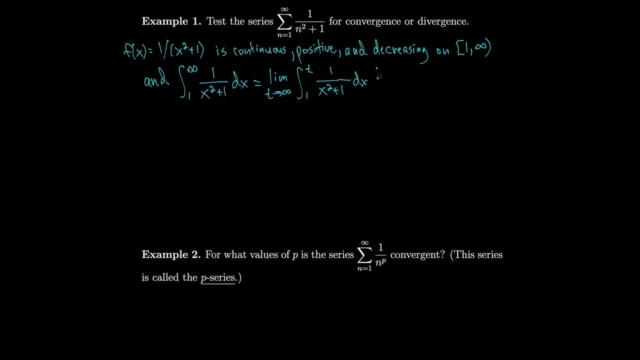 So we take our antiderivative. So that's gonna be the inverse tangent of 1 plus x squared is arctangent when you take the antiderivative. So that means that we're taking the limit of. 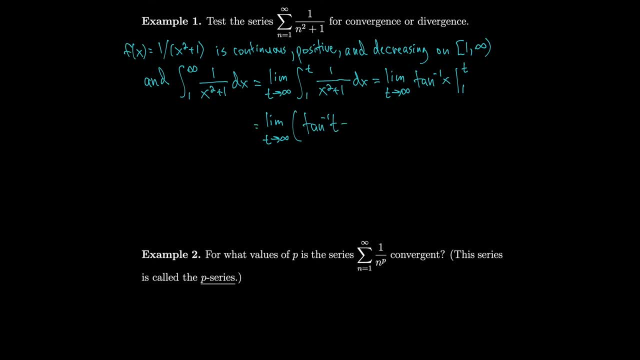 tan inverse of t minus tan inverse of 1, which is pi over 4.. Okay, so remember, as t goes to infinity, for tan inverse of t, we hit an asymptote at pi over 2.. So this limit is pi over 2.. 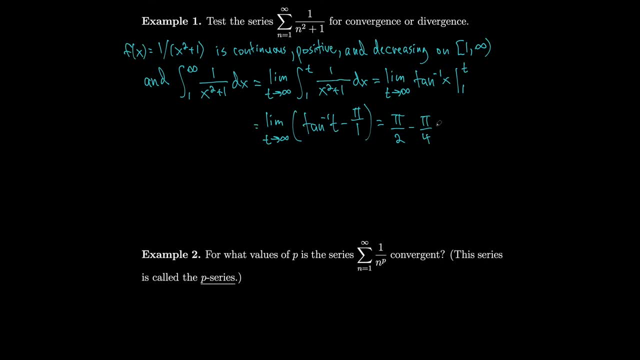 minus pi over 4. which is pi over 4.. So our integral converges. So since our integral converged, that implies that the sum of 1 over n, squared plus 1. also converges, And it's convergent. 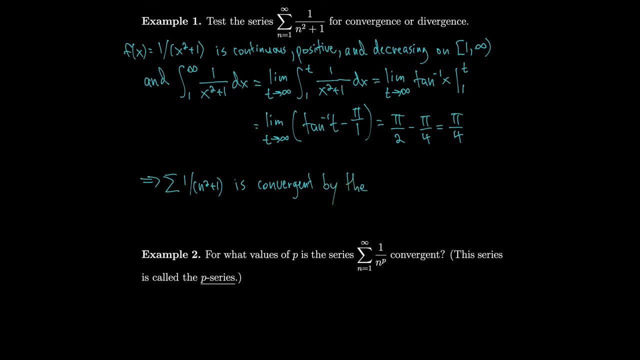 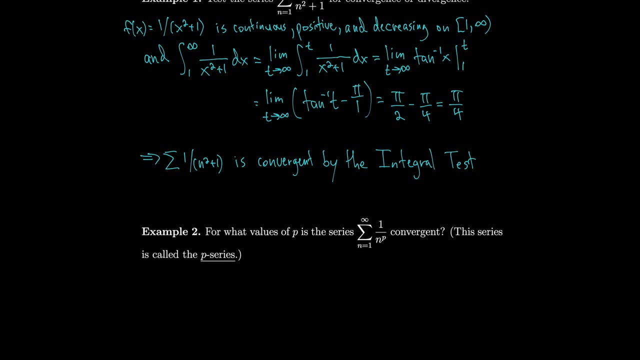 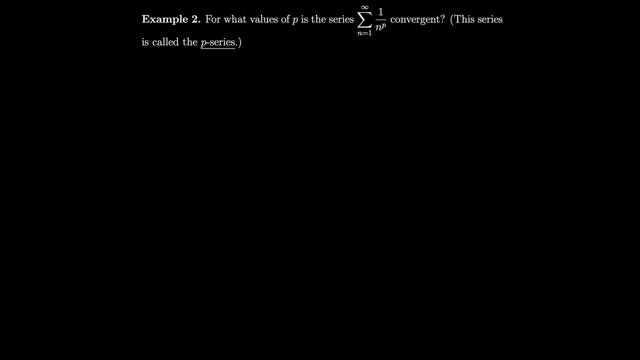 by the integral test. Remember, we did not get the value of the series. We only saw that we could get the value of the series, hopefully potentially using some other method. Let's see if we can figure out what values of p. 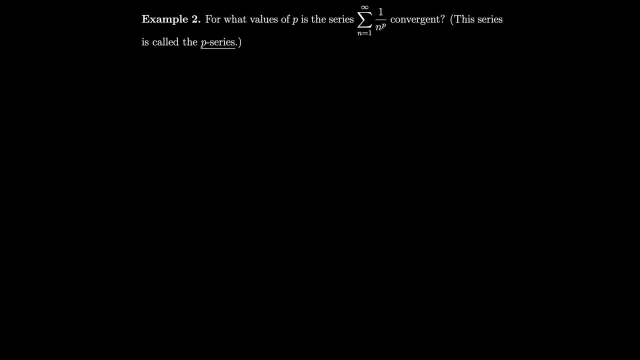 are convergent, p-series is just 1 over n to the p summed up. So let's split it up into different values of p. Notice that if p is negative, then we're looking at the limit of 1 over. 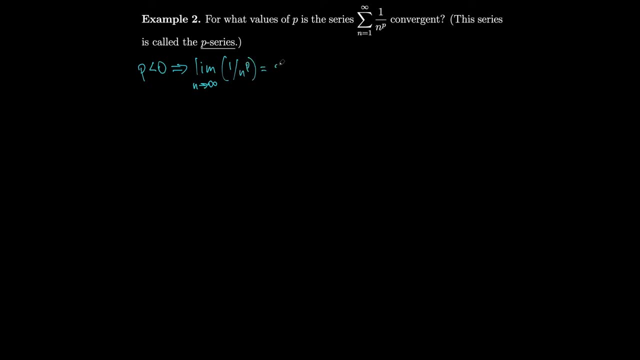 n to the p, And that's infinity. The only reason I'm looking at the limit of 1 over n to the p instead of the limit of the entire partial sum is that we have a test for divergence, or nth term test, which says that if the 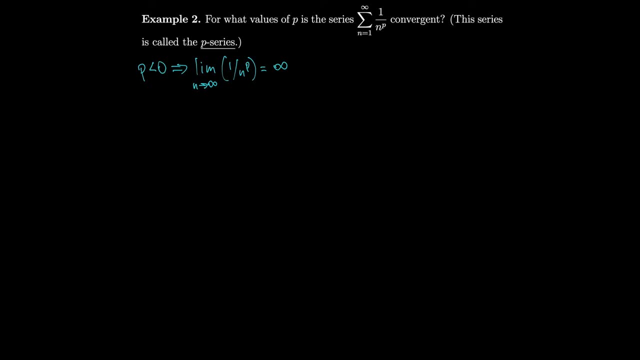 limit of the sequence is not 0, then you can't even bother to try to even take any kind of sum. It's not going to happen. Your sequence has to level off if you want to be able to add anything up. 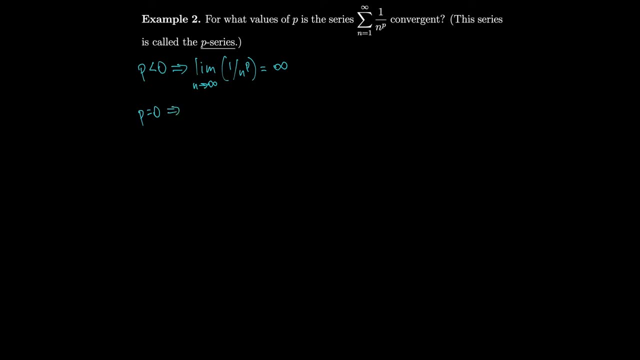 So let's look at: p equals 0. now We have the exact same thing. Our limit of 1 over n to the p becomes the limit of 1 over n to the 0, which is 1.. 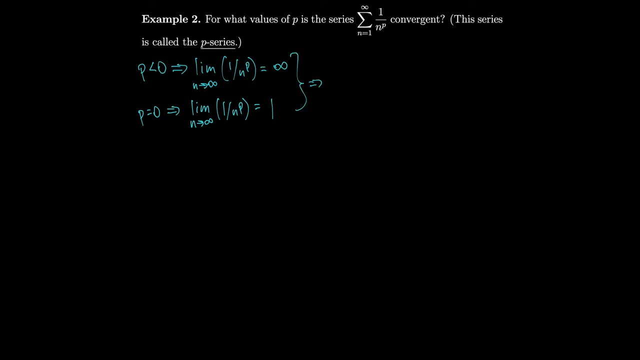 So in both of these cases our sum diverges by the test for divergence. Notice, in the first case, putting a negative value over p is the same thing as really just summing up n to the p, because it's in the denominator. 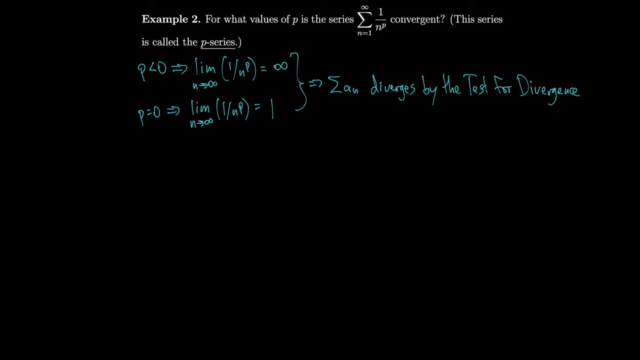 and moves it to the numerator And, summing up, n you know, to some power, over and over and over again. there's no way that could possibly converge. So we saw negative values of p. we saw 0 value of p. 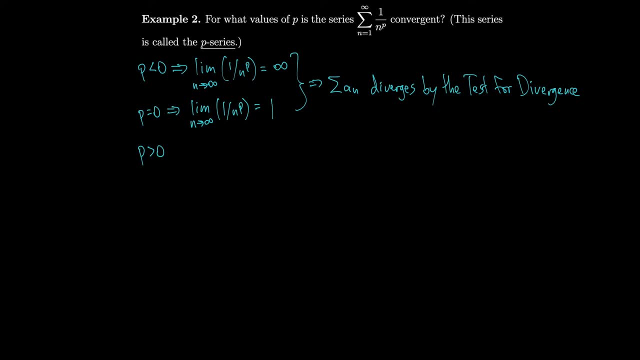 how about we see positive values of p? So if p is positive, then we're going to look at the matching function or corresponding function 1 over x to the p, And that's continuous positive and decreasing. 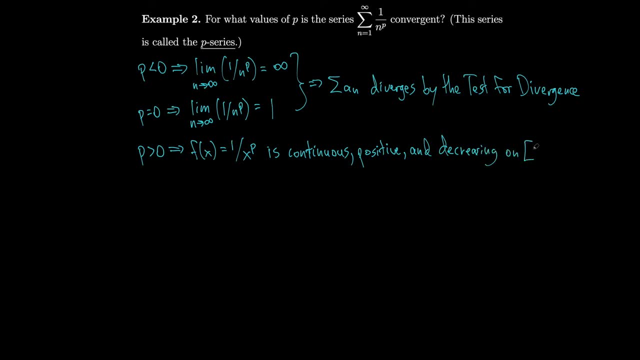 along our interval from 1 to infinity. And if we take a look at our integral of 1 over x to the p, then we know that that converges if p is greater than 1. and it diverges. 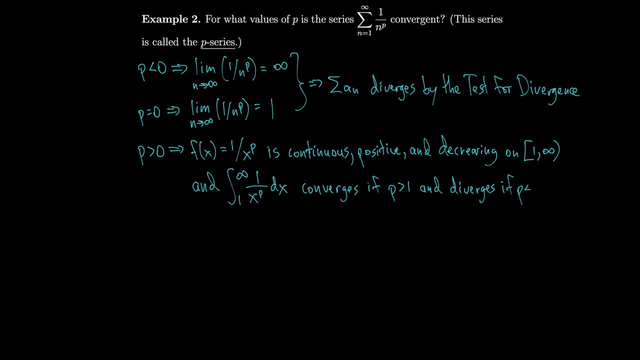 if p is less than or equal to 1.. as we saw in section 7.8.. example 2.. So this means that the sum 1 over n to the p converges if p is greater than 1.. 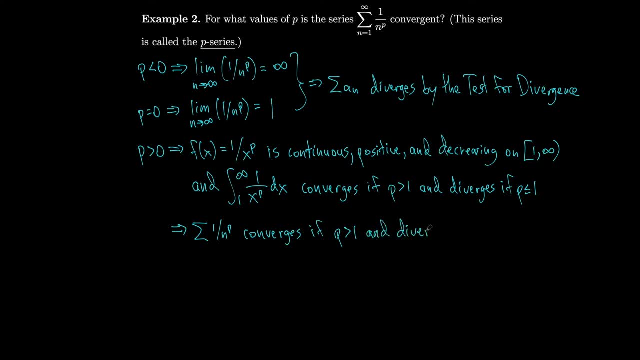 and diverges if p is between 0 and 1.. Notice, if p equals 1, we get the harmonic series, And this is all by the integral test. So we have another kind of proof that the harmonic series diverges. 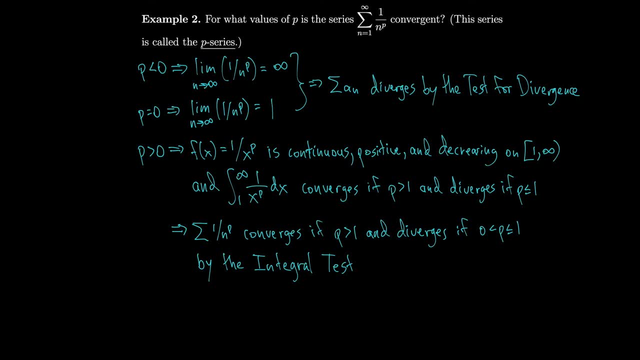 So that means that we only converge if p is greater than 1. because we already saw that it diverges in the other cases by the test for divergence. So how about we summarize all this by saying that our p series 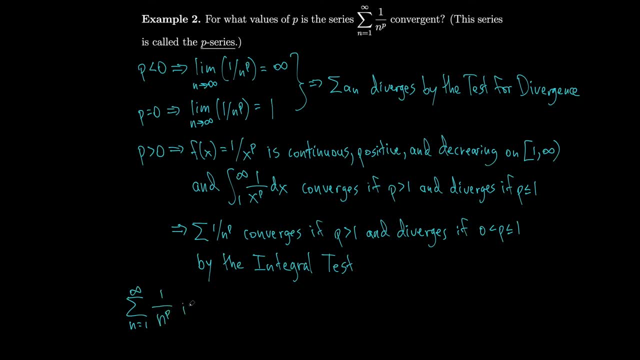 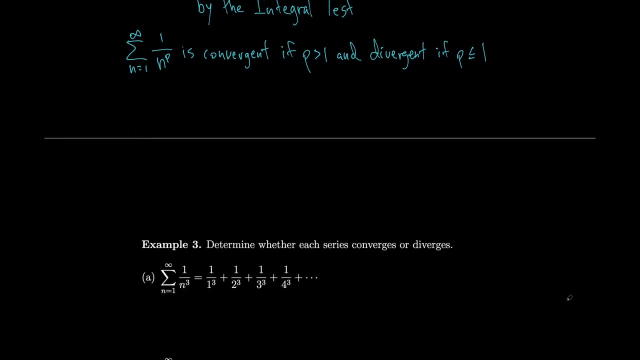 1 over n to the p is convergent if p is greater than 1. and divergent if p is less than or equal to 1.. Let's use what we just proved to see if a couple series converge or diverge. 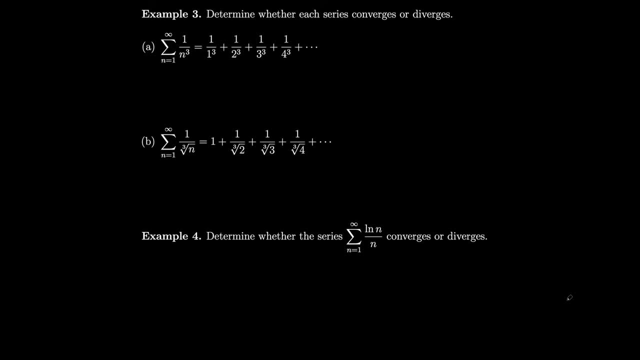 Notice 1 over n is 1 cubed. That's just a p series with p equals 3. which is bigger than 1. So our series converges. Notice that 1 over the cube root of n is just. 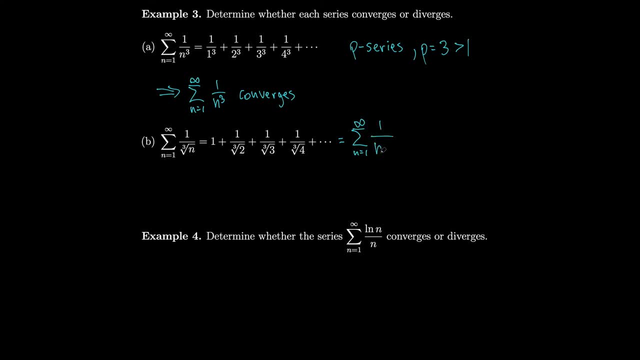 1 over n to the 1 third power. So that's also a p series. In this case, p is equal to 1 third, which is smaller than 1.. So that means that the series diverges because it's a. 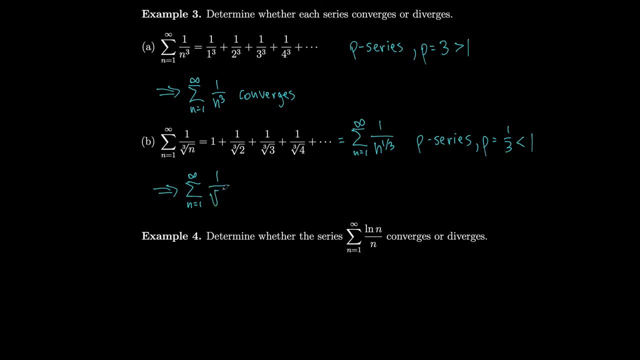 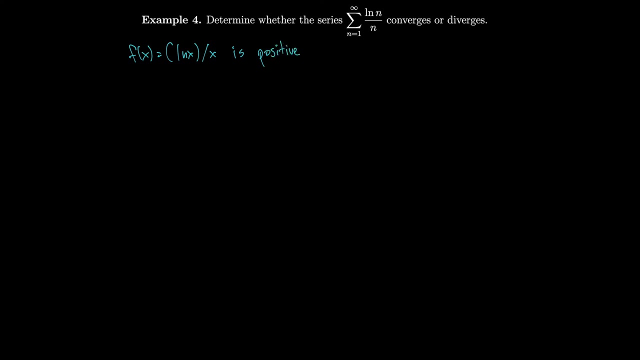 divergent p series. How about this series ln n over n? Well, we have a corresponding function: f of x equals ln x over x, and that's positive and it's continuous for all x values. 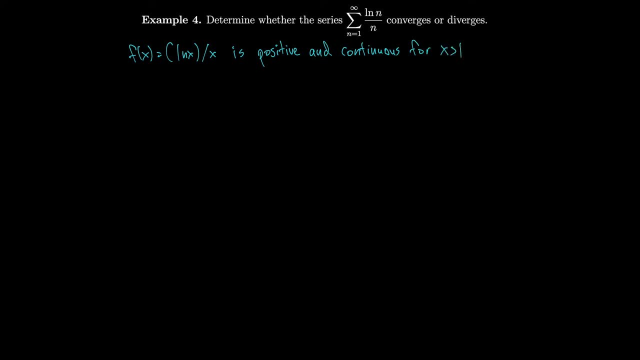 bigger than 1.. However, we don't know if this thing is decreasing at the moment because it's just not so obvious with ln, x over x. So when we want to know if a function is decreasing, we can look at the derivative. 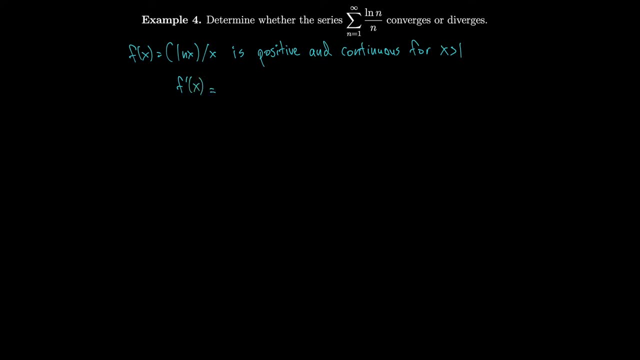 So the derivative can be obtained using the quotient rule. We get 1 over x times x, taking the derivative of ln- x and then minus ln of x times the derivative of x, which is 1.. We divide by x squared. 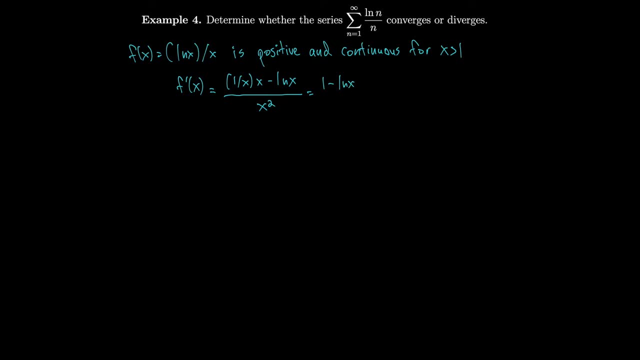 We get 1. minus ln, x over x squared, So that means that this will always be positive. So we only have danger when this thing is bigger than 1. So that means that our derivative will be negative. 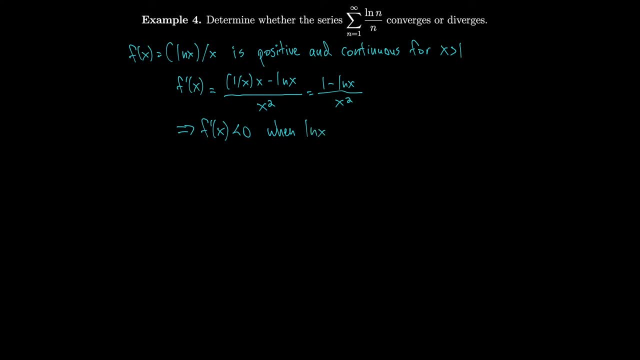 when ln, x is greater than 1.. Which is, when x is greater than e, Just take both sides and raise them to e. So that means that f is decreasing when x is greater than e. So we also have. 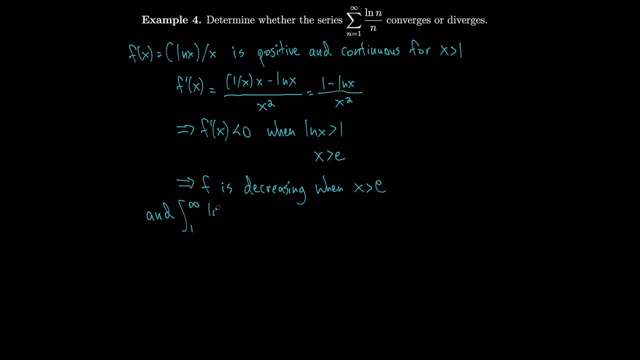 our integral from 1 to infinity of ln x over x, dx is equal to the limit of the integral from 1 to t of ln x over x and taking the antiderivative we get: 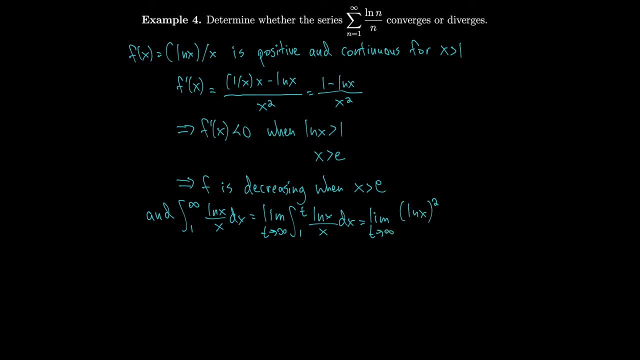 ln, x squared over 2.. and from 1 to t. So that's just the limit of ln, of t squared over 2.. And as t goes to infinity, ln goes to infinity, so our integral is divergent. 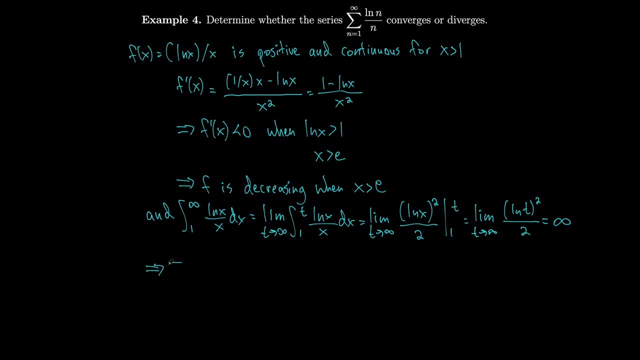 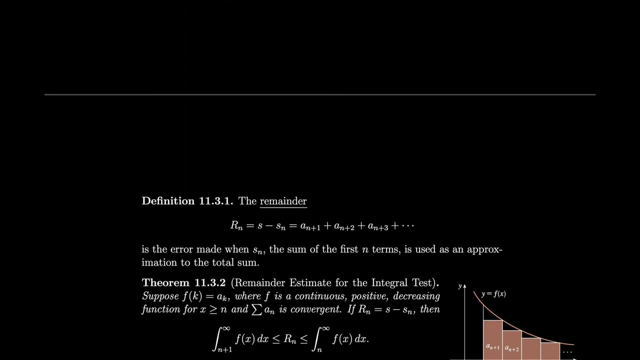 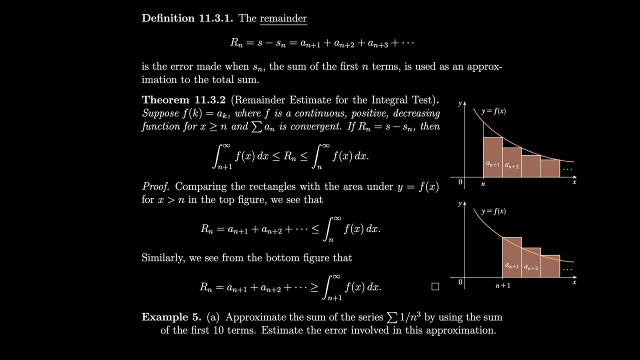 So, since our integral diverges and everything meets up for the criteria for our integral test, we know that the sum of ln over n diverges by the integral test, The remainder s minus sn, which is the sum of our series. 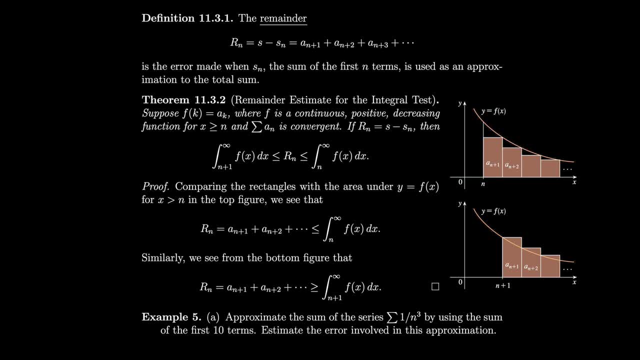 minus the partial sum divided by the sum over n. So if we add up the first 10 terms, then every term after 10.. in our infinite series would be the remainder. So our remainder tells us how far off we are. 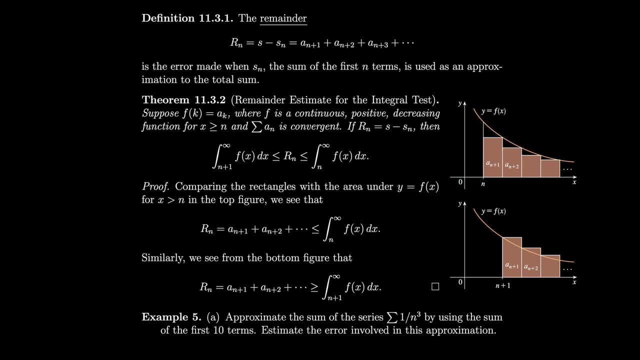 from our actual sum if we use a partial sum to estimate it. So we have a theorem that the remainder is bounded by these two integrals, Provided that of course, you know, is positive and decreasing. so this should sort of make sense, because if we 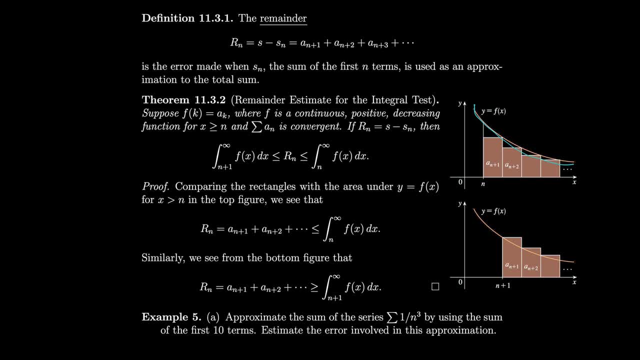 take a look at the integral, then our remainder is just all of these rectangles where we start at n. so there's obviously a whole bunch of other stuff over here that we haven't looked at. that we've already, you know, taken as our sum. so this is everything left. well, by our picture we can see that. 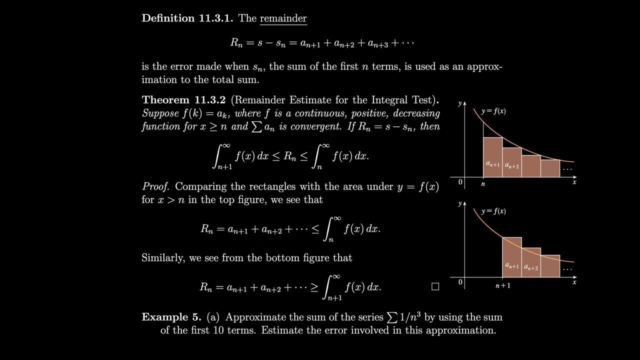 everything left is going to be a n plus 1 all the way on to infinity. that's just the integral from n to infinity. so it should make sense that this is our remainder and it is smaller than the value of the integral. doing the same trick that we did when we prove the integral test, we can take rectangles on. 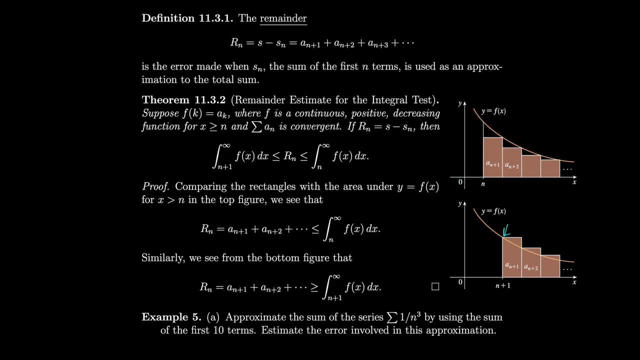 the left side and start at n plus one, and then we'll see that all of these rectangles are also our remainder and they are bigger than the integral, providing that we move the integral down, start at n plus one instead, so that makes sense, that our remainder will be sandwiched in between these two integrals. let's approximate: 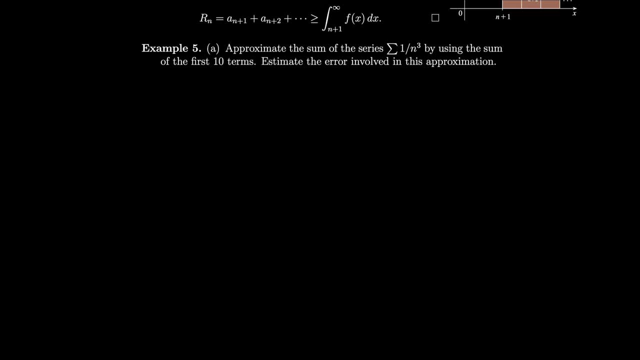 the sum of the series one over n cubed by using the summarizing formula, before we move to simplifying at: in addition to И provides information on how similar integrity of the first 10 terms, and then we can estimate the error involved using our error test. so, in order to 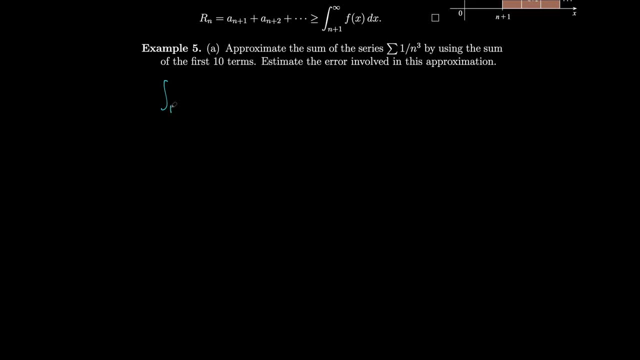 do this, we're going to need the integral at some point, from n to infinity, so might as well compute that. so that's the limit of the integral from 1 over x cubed. so taking the antiderivative, we just get minus 1 over 2x squared and we evaluate that from n to t, basically just skipping the step here. 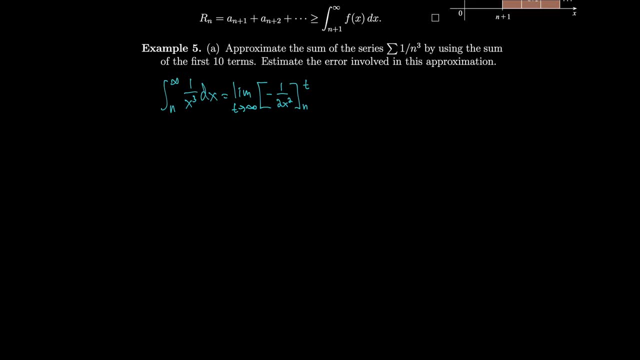 where i replace infinity with t and then jump straight to the antiderivative. so that's just the limit of minus 1 over 2 t squared, plus 1 over 2 n squared, which is 1 over 2n squared. so let's take a look at our sum now. 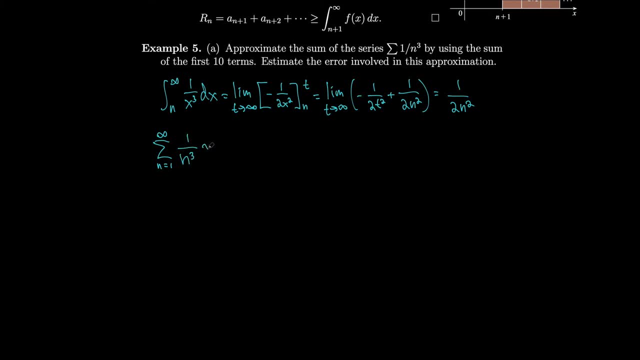 well, that's 1 over n cubed and we want to approximate that using a partial sum up to 10 terms, so that'll be 1 over 1 cubed, plus 1 over 2 cubed, plus 1 over 3 cubed, and so on. 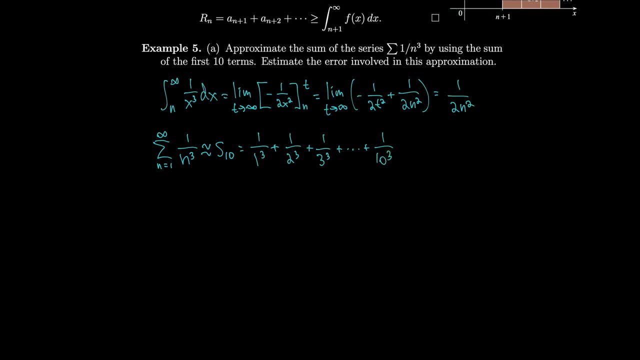 until i've added up the first 10 terms. plugging that into our calculator, we get approximately 1.1975. so this means that our error estimate should be less than or equal to the integral from 10 to infinity of 1 over x cubed. 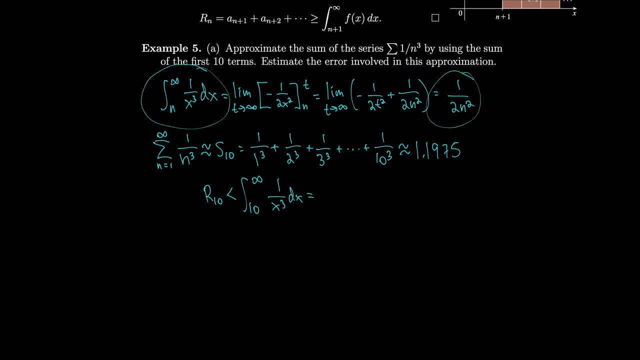 and, as we saw, the integral from n to infinity is just 1 over 2n squared, that this error is going to be at most 1 over 2 times 10 squared, which is 1 over 200.. So this implies that our error is at most 0.005.. 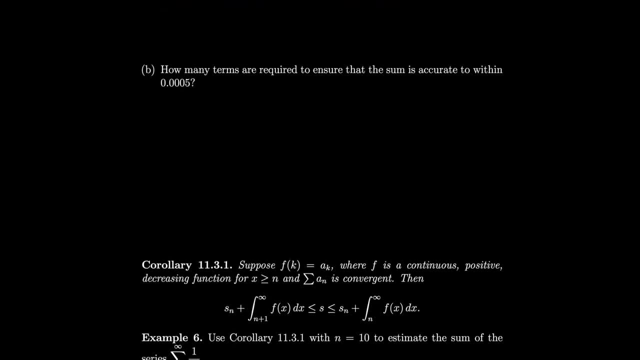 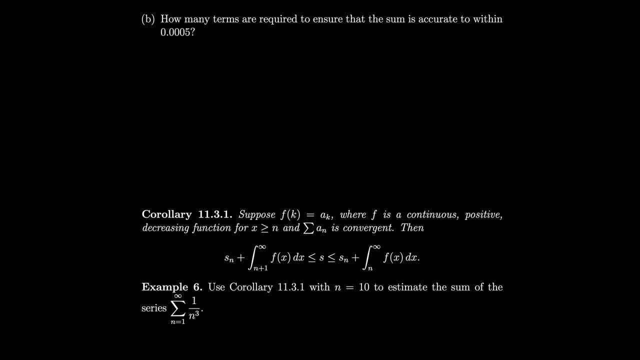 What if we wanted to make our error even smaller? How many terms would we need to have to ensure that the sum is accurate to within 0.0005?? So this means that we want our n, which is less than or equal to the integral from n to infinity of 1. 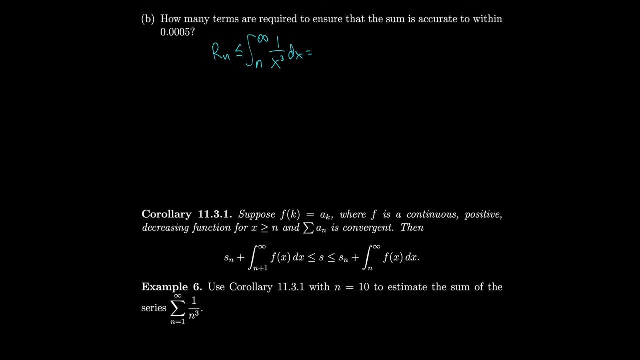 over x cubed, which we saw as 1 over 2n, squared to be less than 0.0005, which is the same as saying that n squared. So that means that n should be greater than 1 over 0.001,. 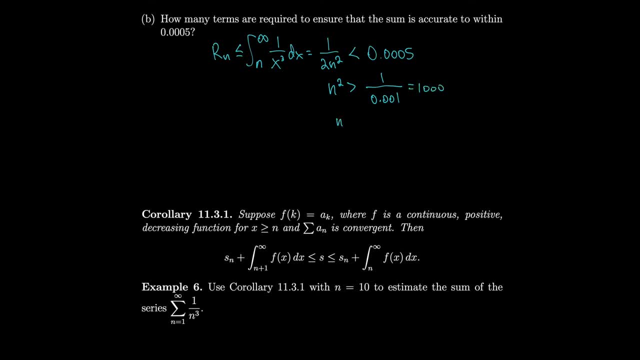 which is 1,000.. So that means that n should be greater than the square root of 1,000, which is about 31.6.. So it looks like we need 32 terms to be on the safe side. This leads us to our next sort of thing. 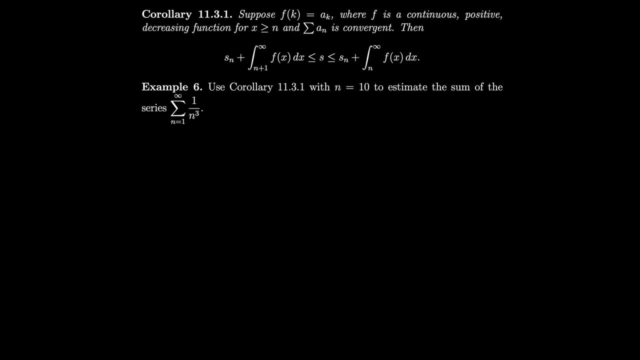 Let's see, Let's see. So we have this sort of problem, which we'll call the S-type theorem, which we'll call the corollary, that if f is a k, where f is a positive, continuous decreasing function- notice, we're using k because we're already 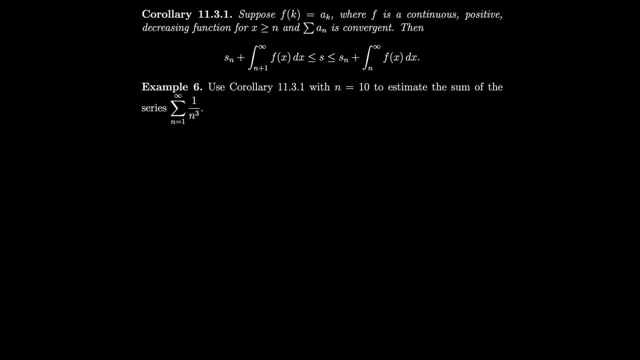 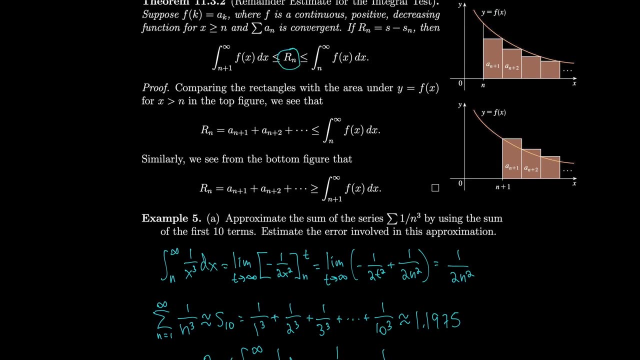 using n, Then if we just take this estimate over here that we had remember, rn is s minus sn. So if I just take s and add it to all three sides, I end up with s by itself over here. I end up with an sn on the left and an sn on the right. 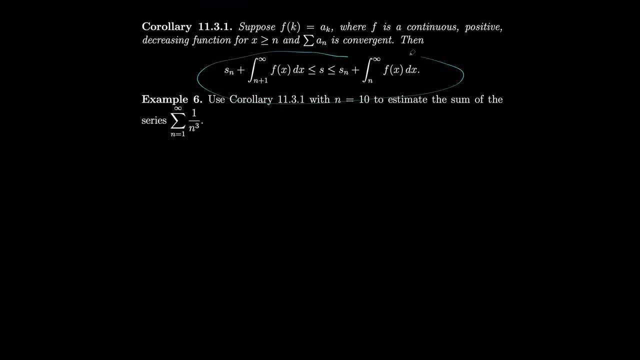 So that gives us this corollary right off the bat. Now we have an integral estimate for our sum of our series. So instead of just estimating a series by cutting off after a certain number of terms and adding up a partial sum, we can. 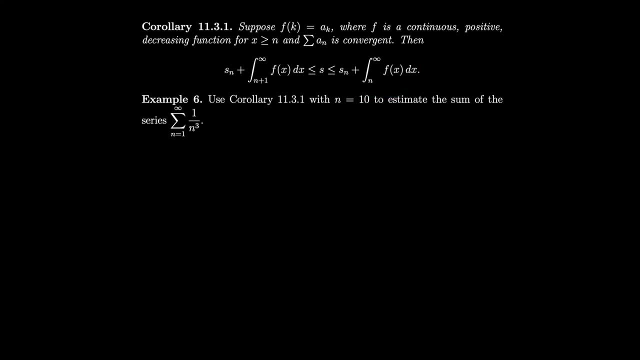 estimate a series using a partial sum added to an integral. So as an example of that, we'll estimate the sum of 1 over n cubed with n equals 10 using this corollary. So we have s10 plus the integral, from n plus 1 to infinity. 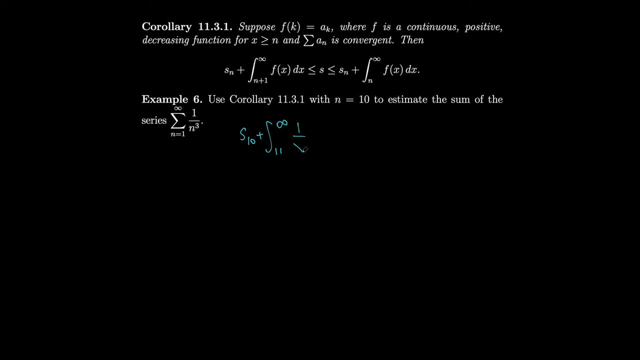 So that's 11 to infinity of 1 over x cubed dx. That must be less than or equal to the actual sum of the series, which is less than or equal to s10 plus the integral from 10 to infinity of 1 over x cubed. 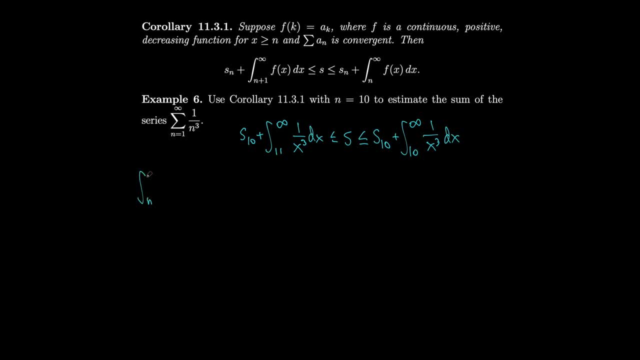 So we already know that the integral from n to infinity of 1 over x cubed is 1 over 2n squared. So that means that s10 plus 1 over 2 times 11 squared, That is less than or equal to s, which is less than or equal. 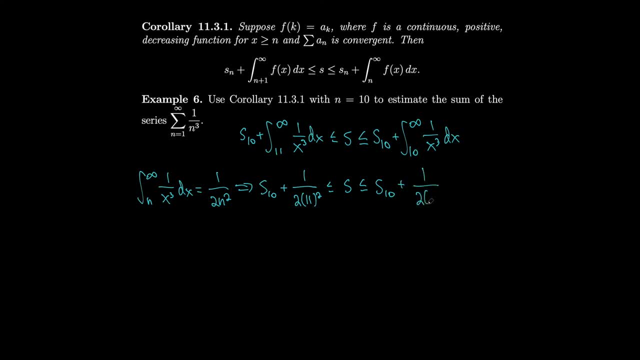 to s10 plus 1 over 2 times 10. squared, As we saw before, our sum of our first 10 terms is about 1.197532.. Just go a couple more decimal places And that means that we have s10 plus 1 over 2. 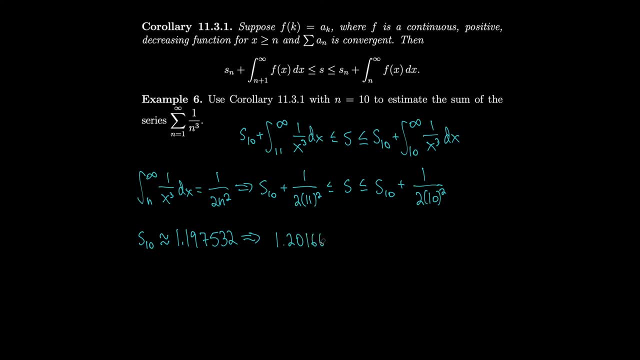 is 1.201664 and our other estimate is 1.202532.. So if we take the middle of this interval and use that as our estimate, then we can say that the sum of 1 over n cubed is about 1.2021.. Since we're in the middle of our 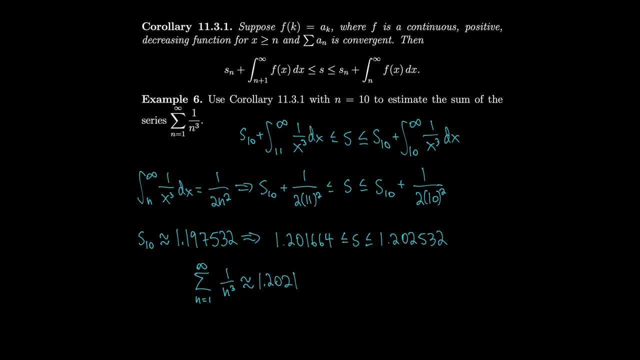 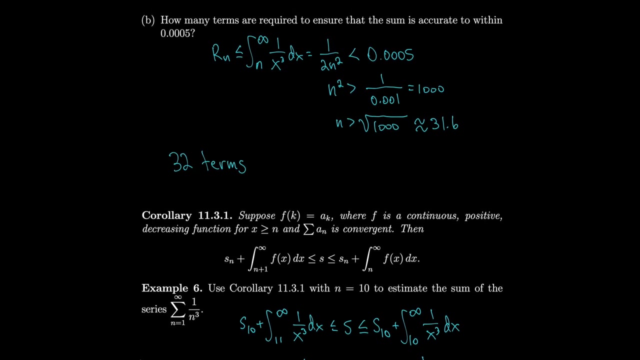 interval. that means that we're halfway between the left and the right. so if we take the width of the interval and divide it by 2, then we see our maximum error is less than 0.0005.. Notice that in order to get to this amount of error, this accuracy, before when we